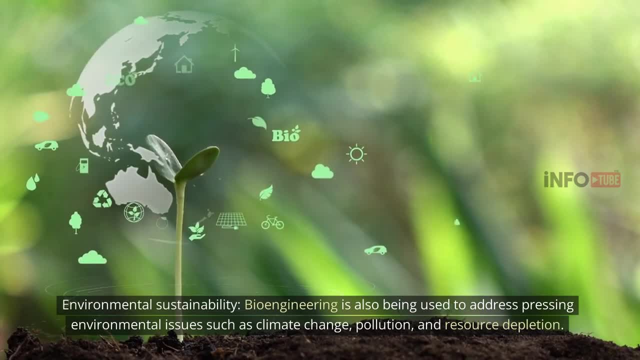 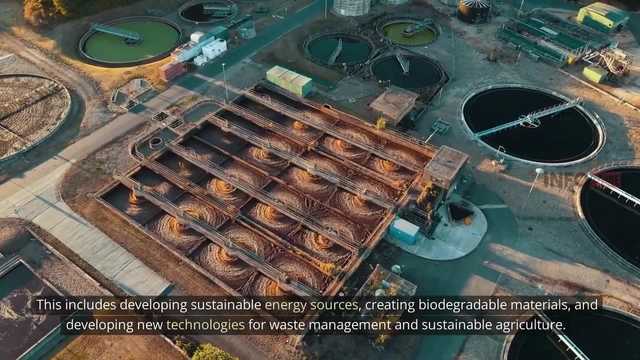 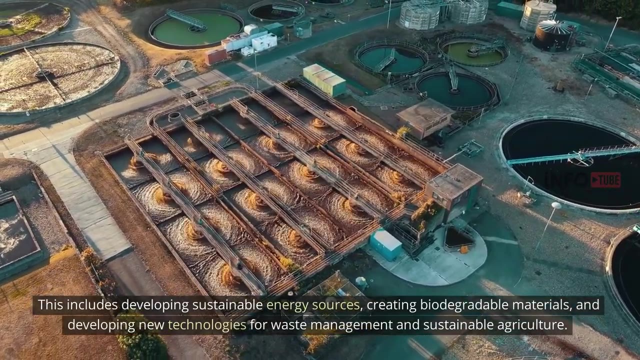 Environmental Sustainability. Bioengineering is also being used to address pressing environmental issues such as climate change, pollution and resource depletion. This includes developing sustainable energy sources, creating biodegradable materials and developing new technologies for waste management and sustainable agriculture. Food production: Another area where bioengineering is making. 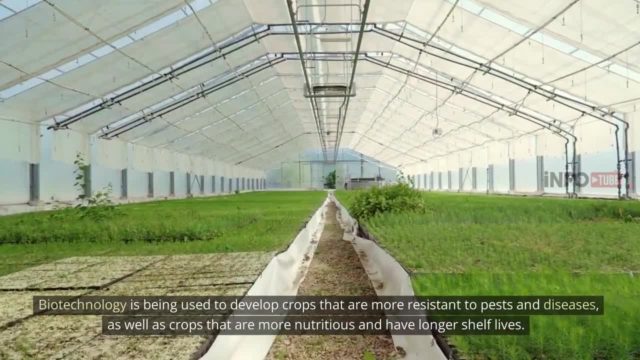 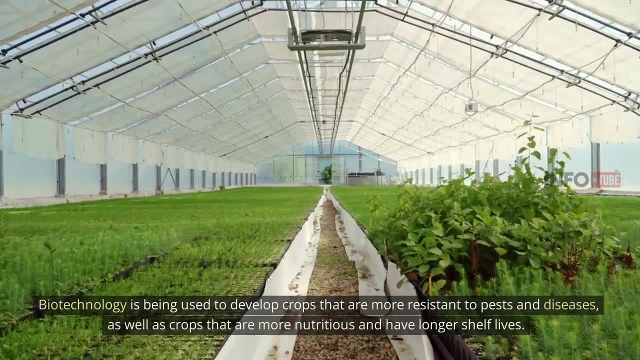 a big impact is food production. Biotechnology is being used to develop crops that are more resistant to pests and diseases, as well as crops that are more nutritious and have longer shelf lives. This includes genetically modified crops and livestock, as well as new techniques for plant. 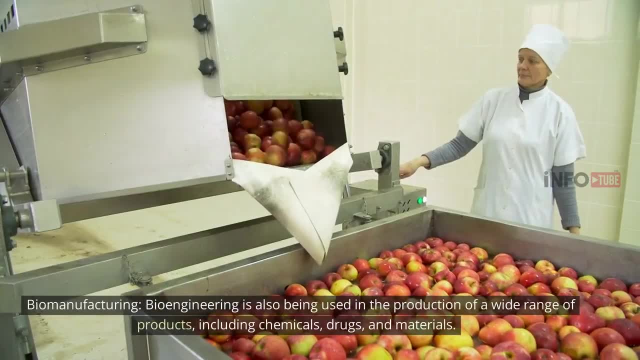 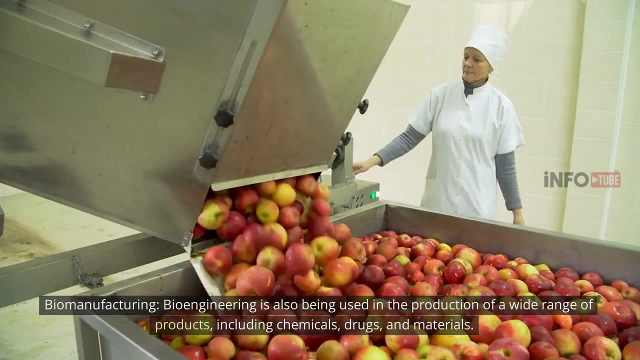 breeding and bioreactor production of food. Industrial innovation is another force of good food. Biomanufacturing- Bioengineering- is also being used in the production of a wide range of products, including chemicals, drugs and materials, By using living systems to produce these products. 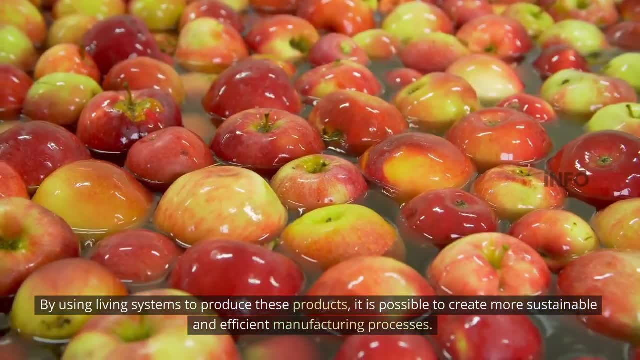 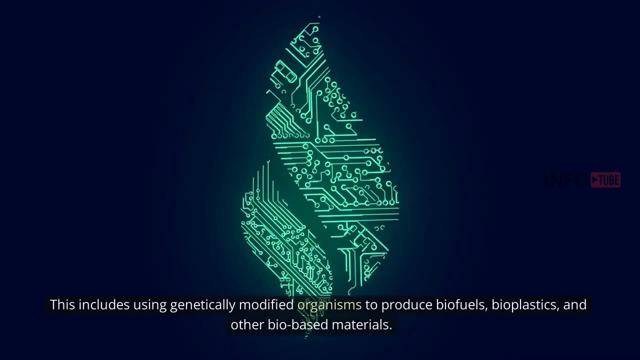 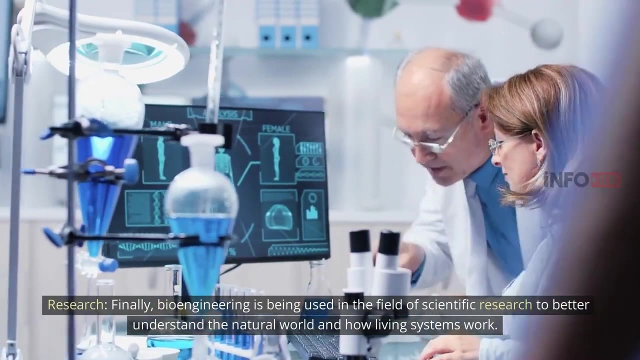 it is possible to create more sustainable and efficient manufacturing processes. This includes using genetically modified organisms to produce biofuels, bioplastics and other bio-based materials. Research, Finally, bioengineering is being used in the field of scientific research to better understand the natural world and how living systems work. 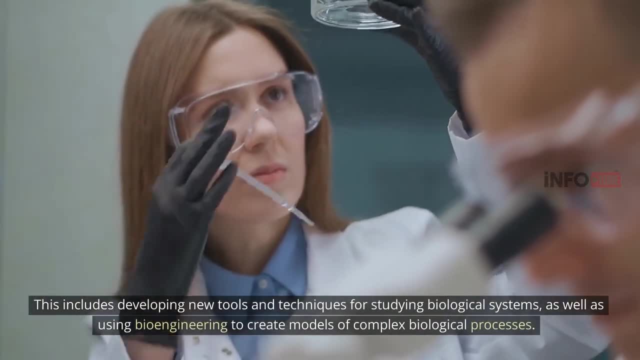 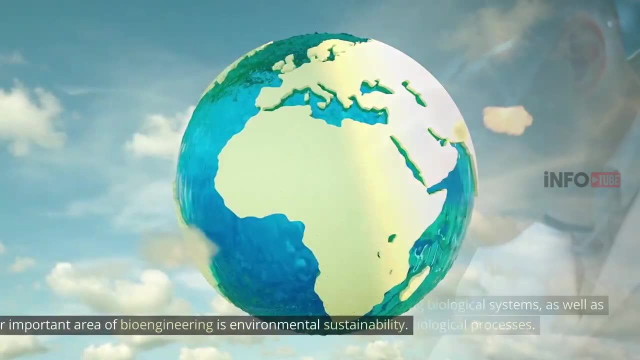 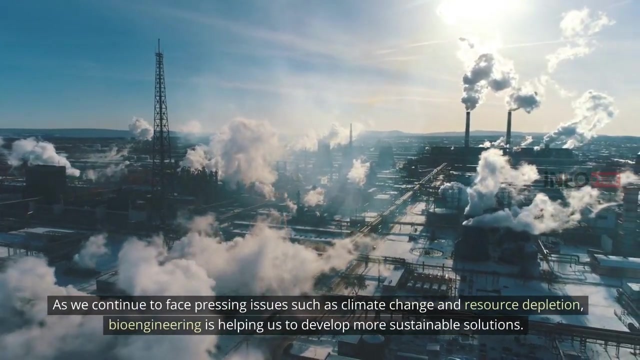 This includes developing new tools and techniques for studying biological systems, as well as using bioengineering to create models of complex biological processes. Another important area of bioengineering is environmental sustainability, As we continue to face pressing issues such as climate change and resource depletion. 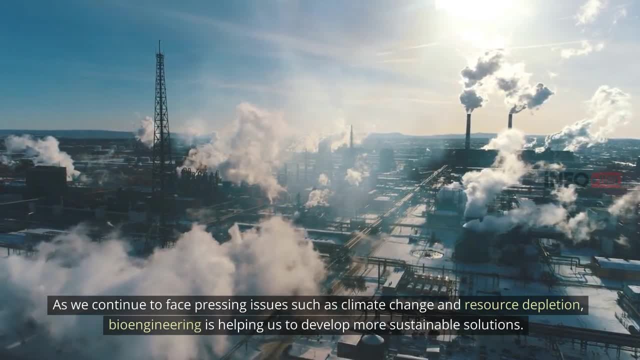 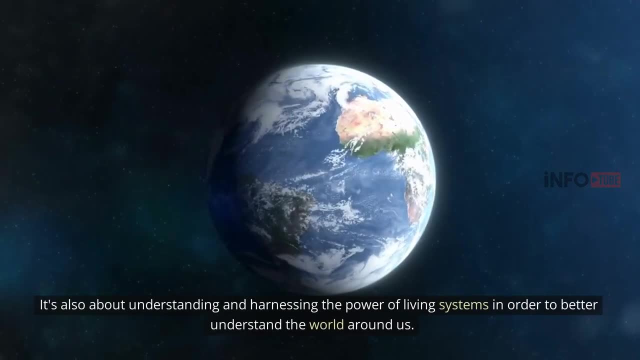 bioengineering is helping us to develop more sustainable solutions. But bioengineering isn't just about developing new technologies. It's not just about creating new technologies and products. It's also about understanding and harnessing the power of living systems in order to better understand the world around us. 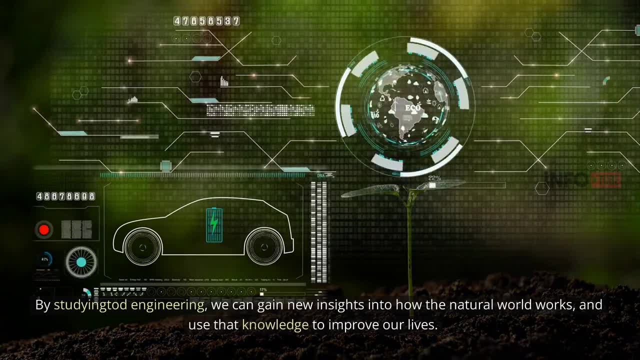 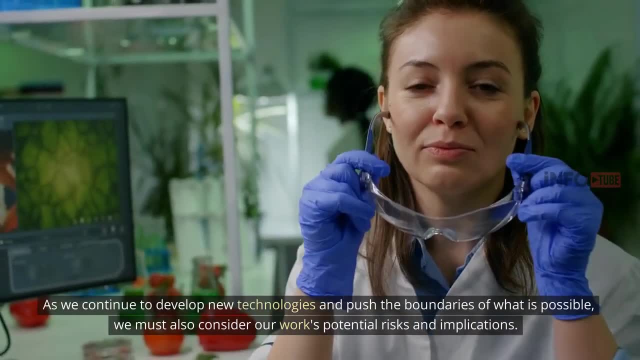 By studying Todd Engineering, we can gain new insights into how the natural world works and use that knowledge to improve our lives. As we continue to develop new technologies and push the boundaries of what is possible, we must also consider our work's potential risks and 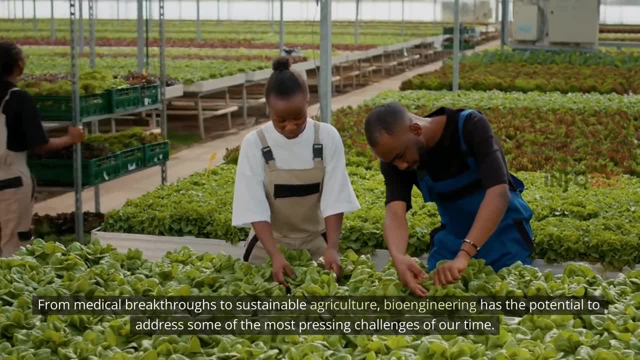 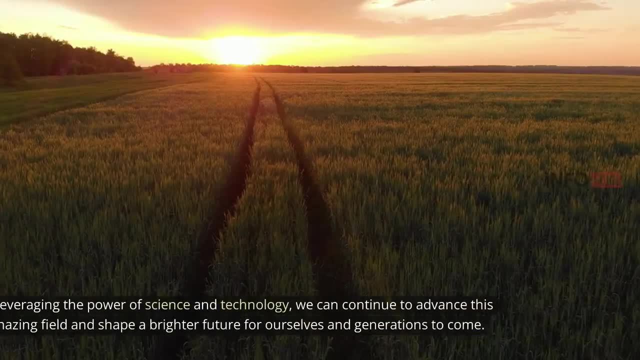 implications, From medical breakthroughs to sustainable agriculture. bioengineering has the potential to address these challenges. Bioengineering is being used to develop new technologies to address some of the most pressing challenges of our time. By leveraging the power of science and technology, we can continue to advance this amazing field and